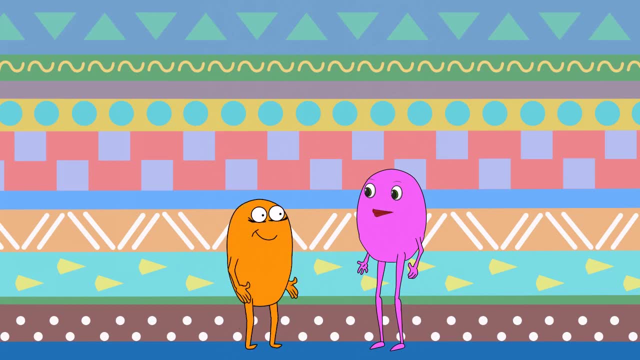 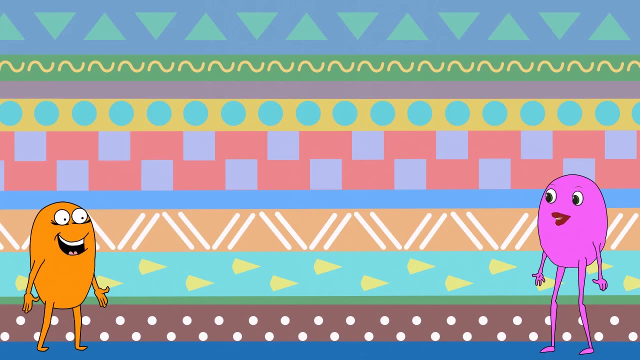 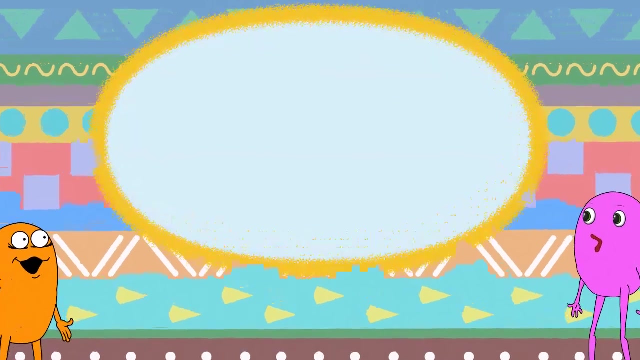 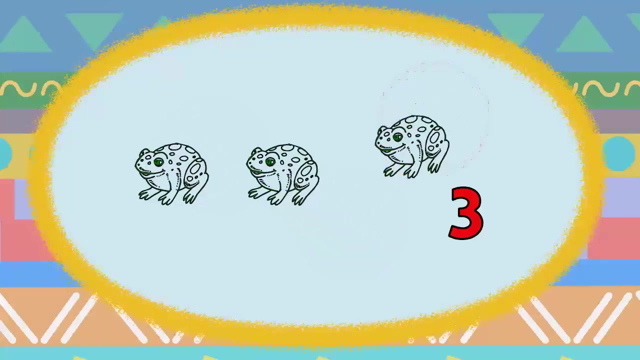 Are you ready to play? Molly? Yeah, Bring on the counting. Bring on the counting. I know how Let's go. I know numbers now: One, Two, Three, Three frogs. Way to go. Molly, One, Two. 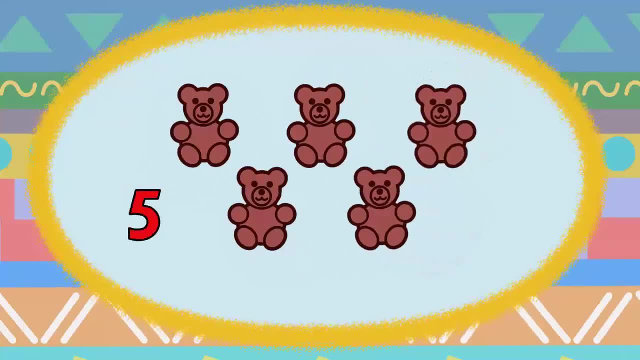 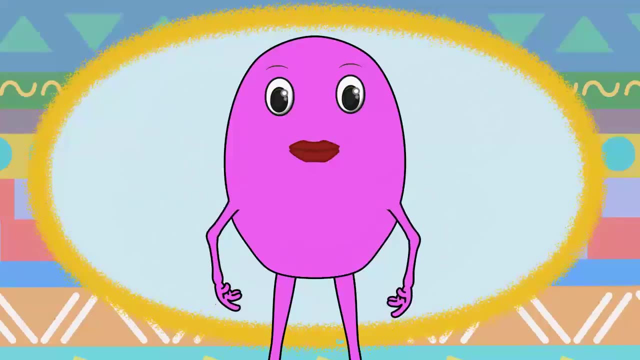 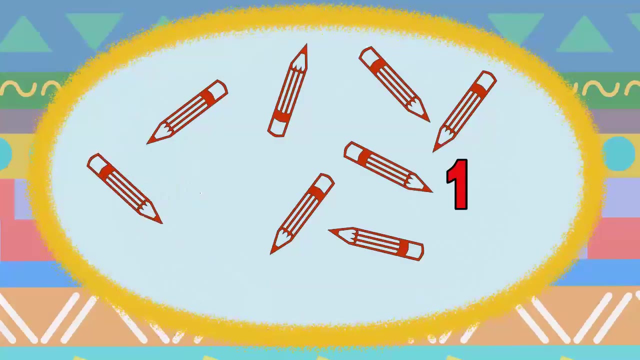 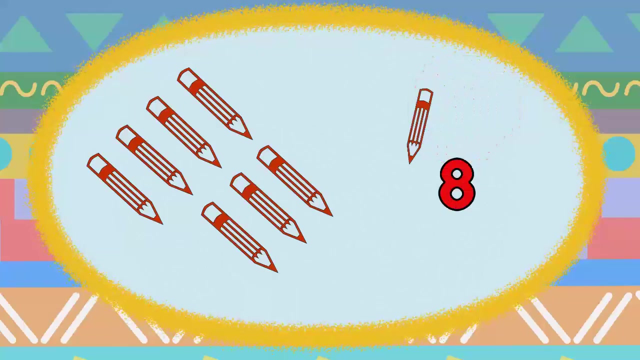 Three, Four, Five, Five teddy bears. Now let's count together. Come on, kids, Count along with us. One, Two, Three, Four, Five, Six, Seven, Eight, Eight pencils- Shut up, man. 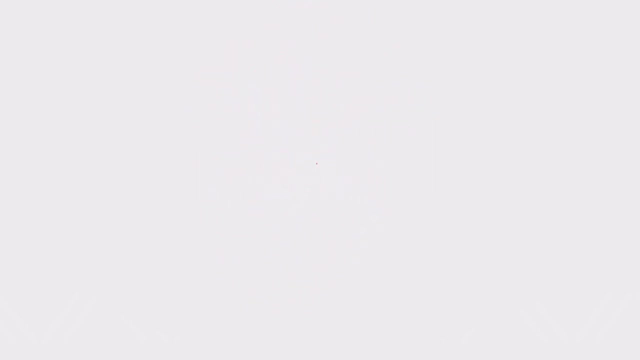 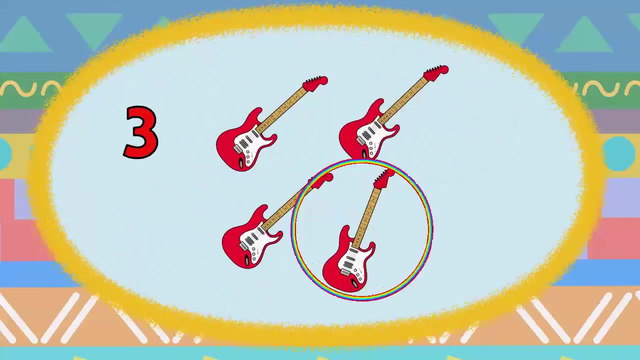 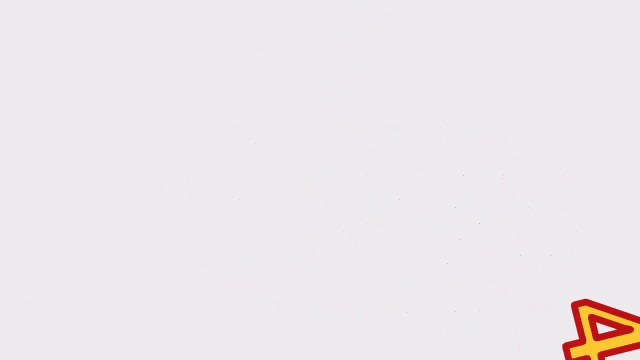 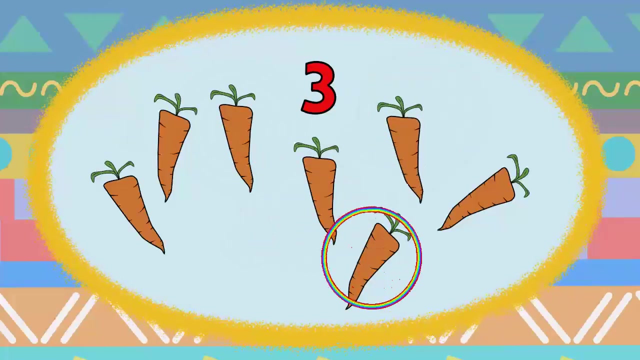 I was just you know playing a little bit of how to play: One, two, three, four, five, six, seven, eight Eight pencils: One, two, three, four, four guitars: One, two, three, four, five, six, seven. 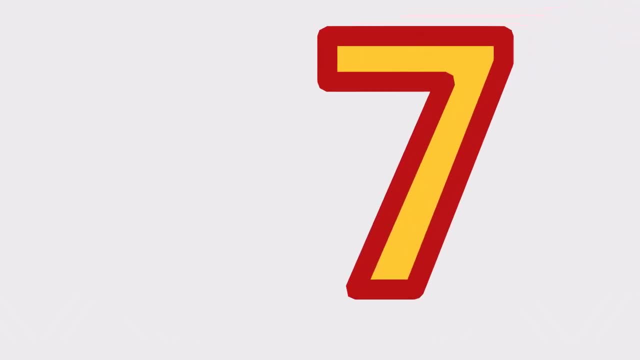 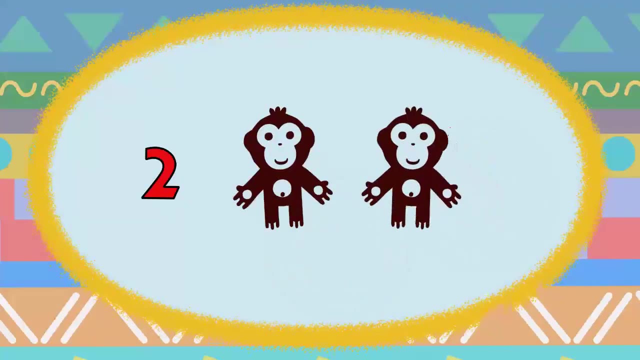 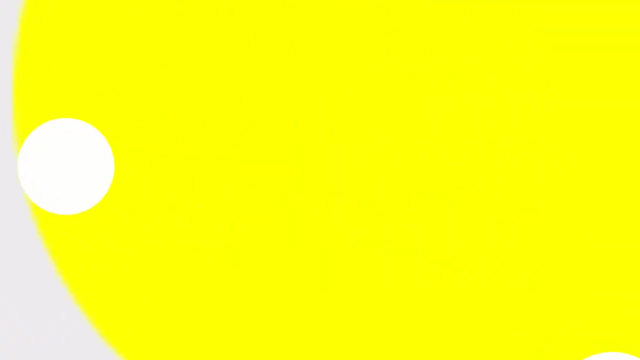 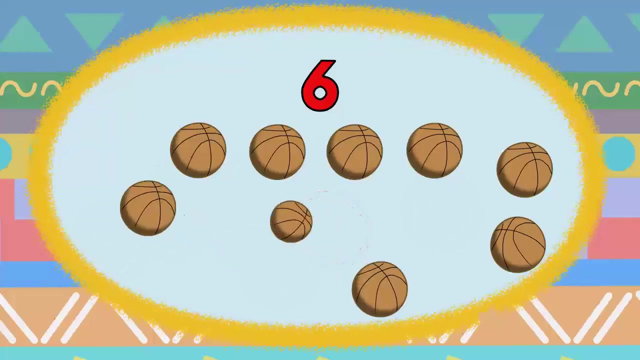 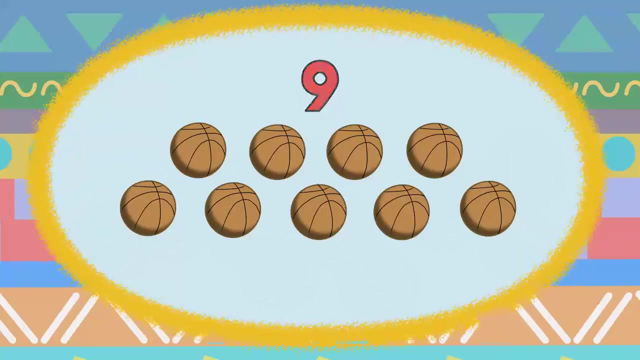 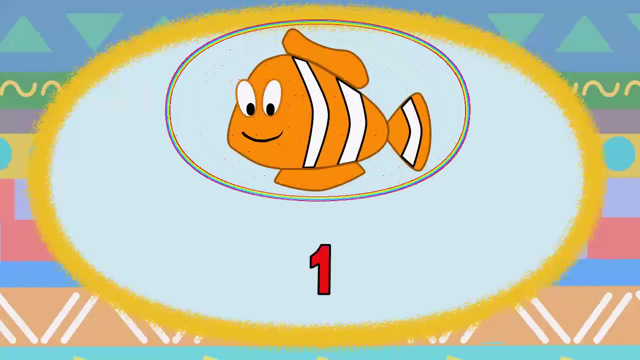 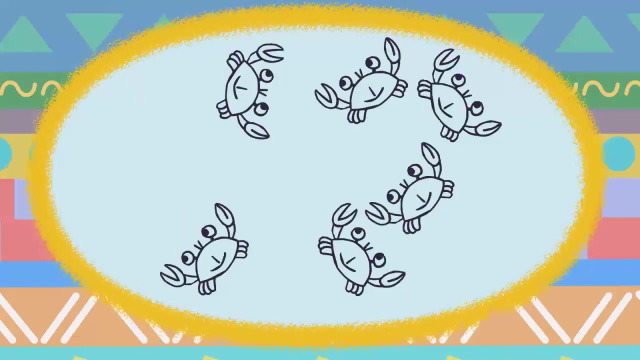 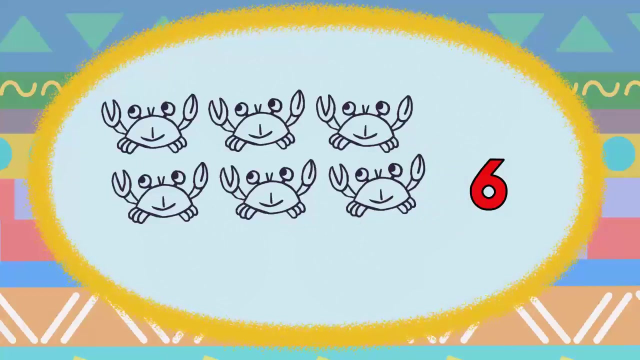 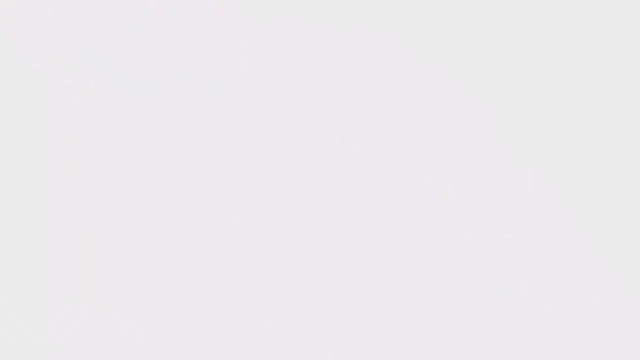 Seven carrots, One, two, two monkeys. One, two, three, four, five, six, seven, eight, nine Nine basketballs: One, uh, just one. One fish. One, two, three, four, five, six, six crabs.